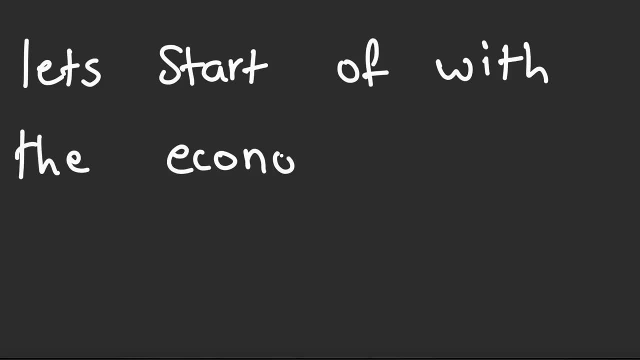 All of IGCIC economics in nine minutes. Let's start off with the economic problem. The economic problem is simply: when we have fewer resources and unlimited ones, We need to know two types of goods: the economic goods and the free goods. Well, the economic goods have opportunity costs. 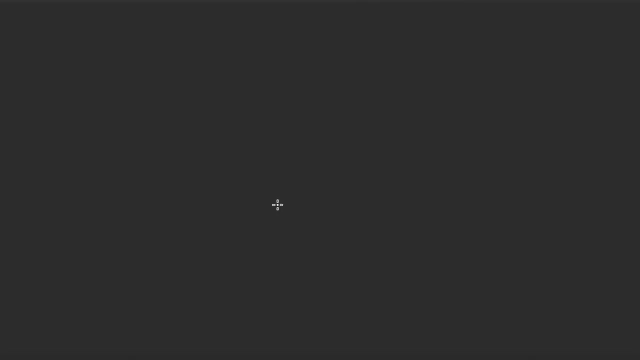 and the free goods do not have opportunity costs. An example is sunlight. We have four factors of production. You can remember this- with cell capital, enterprise land and labor, Land being the natural resources used in the production. Labor is the human resources used in the production. 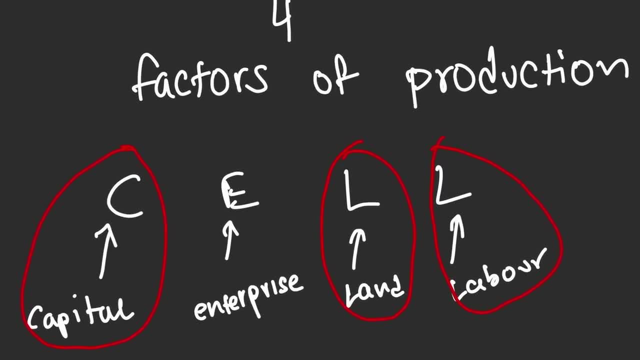 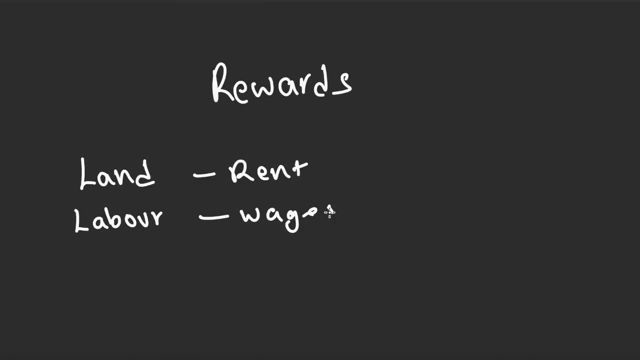 Capital is the manufactured resources that are used to produce these goods and services, And enterprise is the skills and willingness of a person to take risks. The rewards for the factors of production is: land is rent, labor is wages, capital is interest and enterprise is. 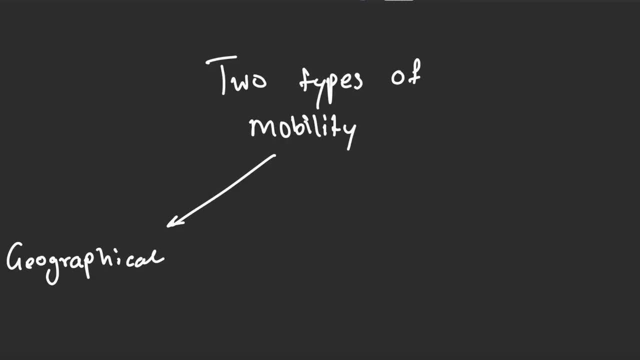 profits. We have two types of factors of mobility and that is geographical mobility, which refers to the willingness of someone to relocate due to employment purposes, And the reasons of this could be the family ties, related commitments and cost of living are reasons why they would not want. 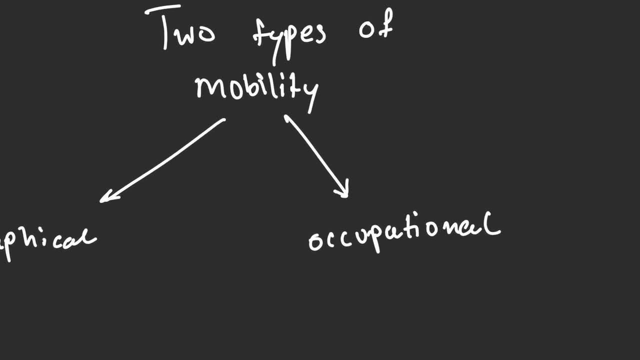 to relocate. Occupational mobility is simply when it refers to someone changing jobs, and this could vary according to cost, Training period and educational profession. Looking at opportunity cost, opportunity cost is the cost of the next best alternate of choosing a good and you can represent the opportunity cost. 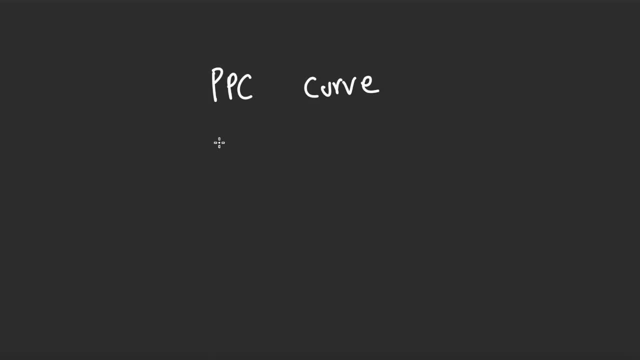 with a production possibility curve. You need to understand the points in the production possibility curve. If the point is inside, it is inefficient. If the point is outside, it is unattainable With the movements of the PPC curve. if it's an outward shift, that means you have discovered raw. 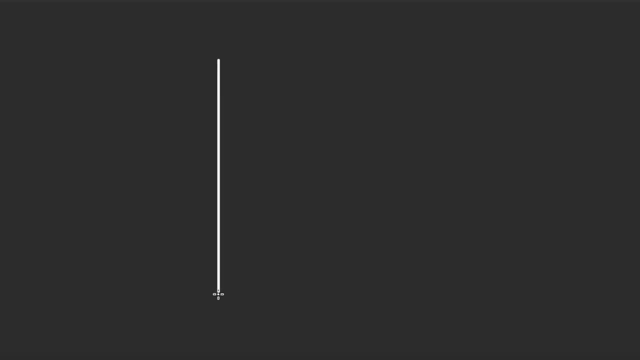 materials, new technology, increase in the labor force. If it's an inward shift, that means there's natural disasters, very low investments in technologies and running out of resources. Moving on, economics is divided into two: microeconomics and macroeconomics With. 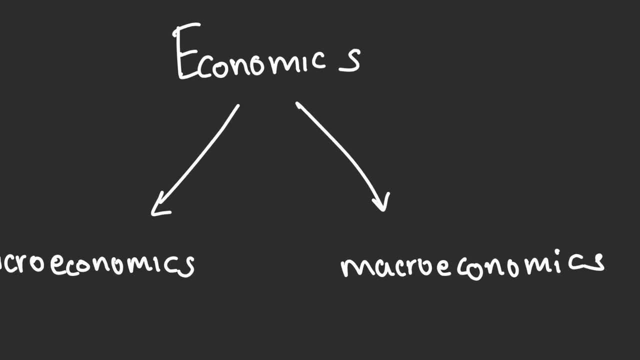 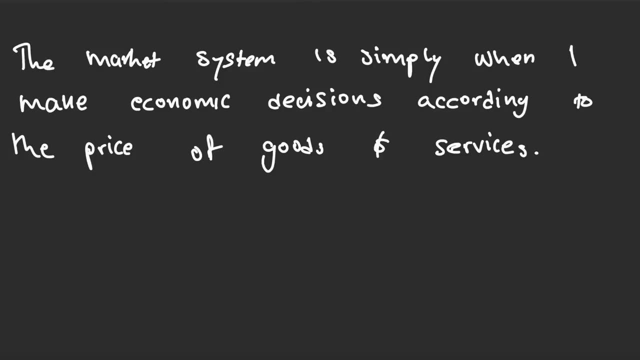 microeconomics, we study particular markets, while with macroeconomics, we study the whole economy. The market system is simply when I make economic decisions according to the price of goods and services that are dependent on the supply and demand. What are the three key questions of 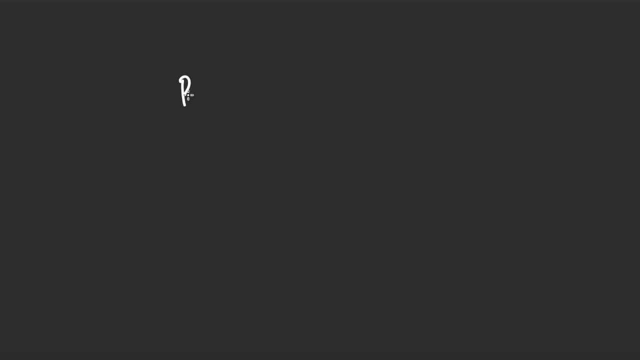 economics: what to produce, how to produce and for whom to produce. The price mechanism is simply when I make a decision according to the equilibrium point where the supply and demand curve meet. What is demand? Demand refers to the willingness and ability of customers to buy goods and services at a given 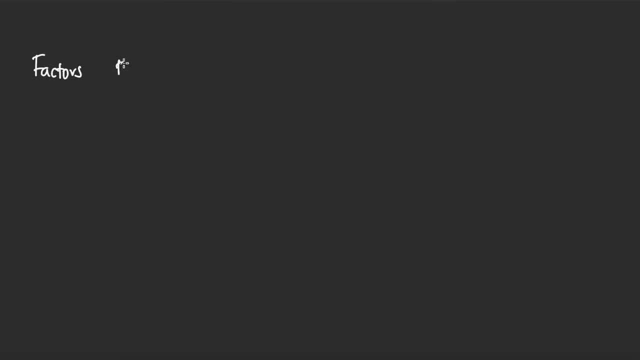 price. The higher the price of a good, the less the demand. Factors that affect demand are price, advertising, government policies, consumer tastes, consumer income, price of substitutes, interest rates. Individual demand is demand of one individual or firm and market demand. 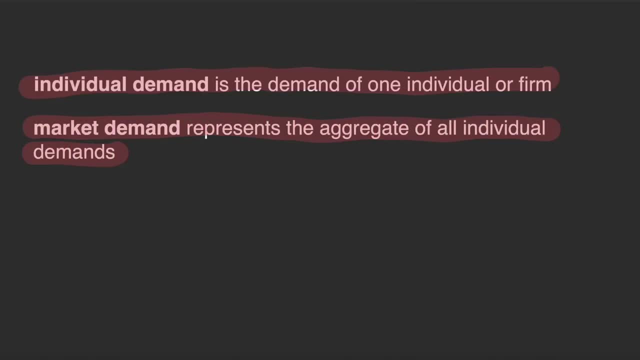 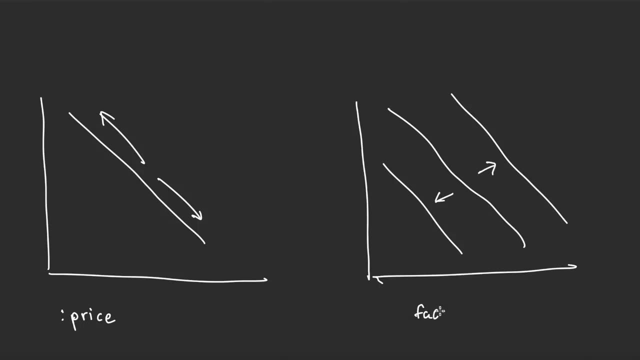 represents the aggregate of all individual demands. Movement along the curve is due to change in price in the demand curve and shift of the curve either right or left is according to the factors of demand. Supply refers to the ability and willingness of suppliers to provide goods and 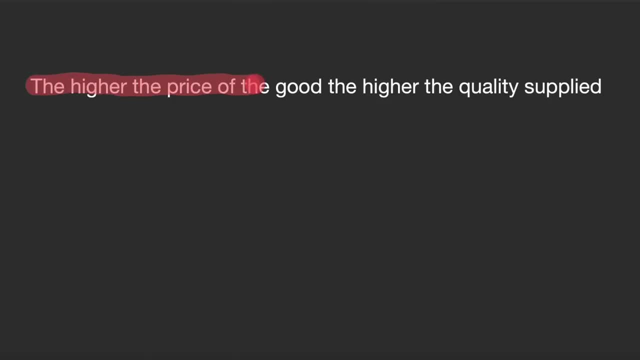 services at a given price. The higher the price of the good, the higher the quantity supplied. The factors that affect supply are cost of factors of production, prices of other goods, global factors, technology advances and business optimism. The individual supply is the supply of: 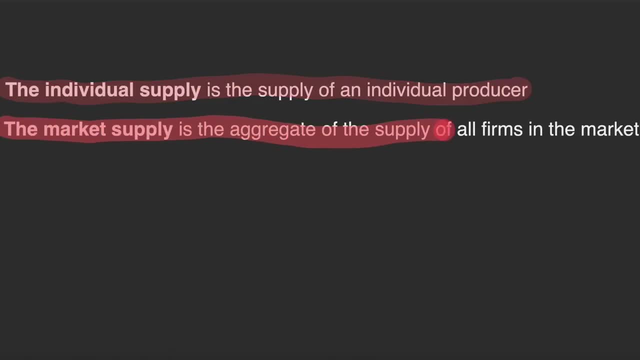 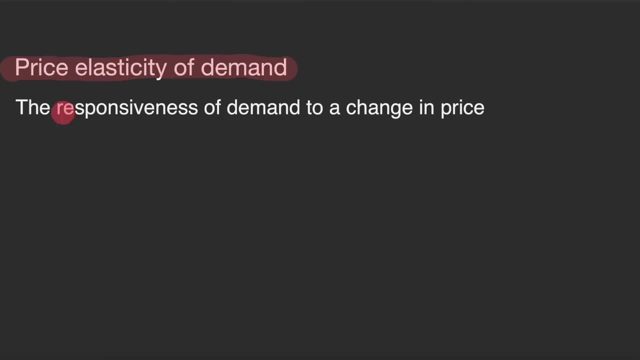 an individual producer. The market supply is the aggregate of supply of all firms in the market. Market equilibrium is when the supply and demand are equal in an economy. Then we have the price of demand, which is simply the responsiveness of demand to the change in price. We have inelastic. 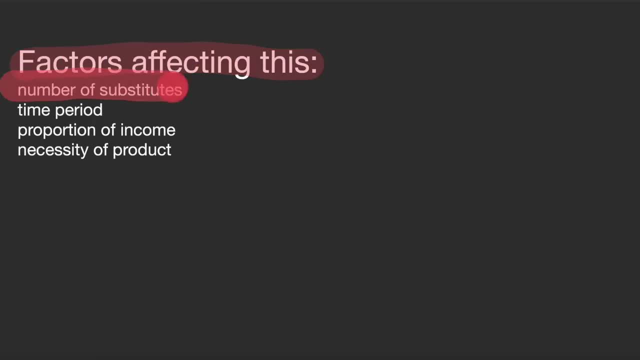 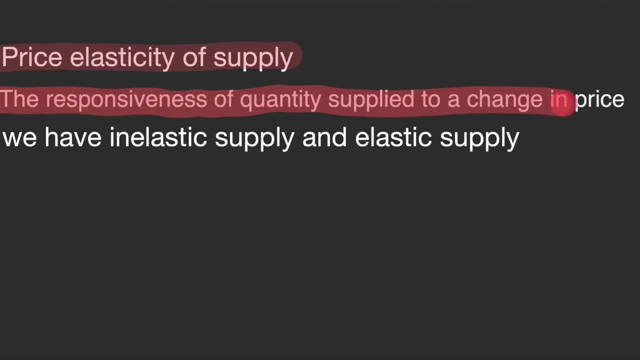 demand and we have elastic demand. The factors that affect this is the number of substitutes, the time period, the proportion of income and the necessity of the product. With price elasticity of supply, it's the responsiveness of quantity supplied to a change in price. We have inelastic. 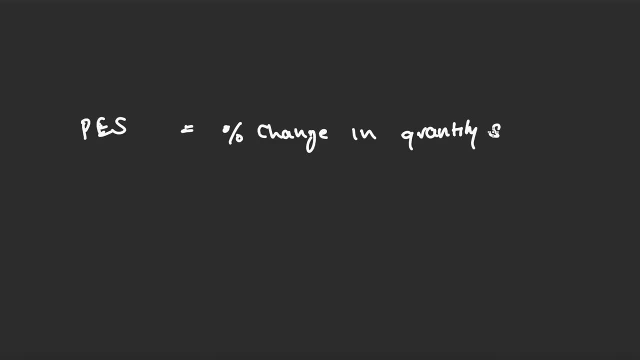 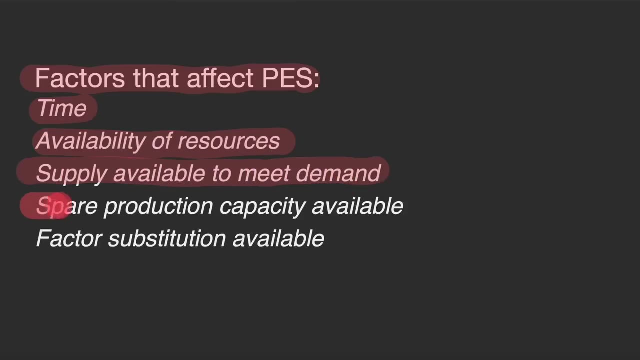 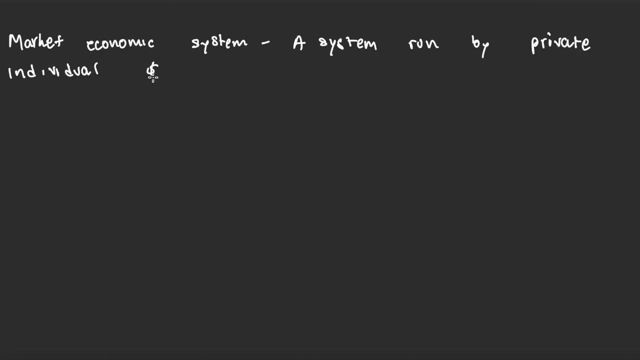 supply and elastic supply. The formula for this is percentage change in quantity supplied over percentage change in price. Factors that affect PES are time availability of resources, supply available to meet demand, spare production capacity available and the factor substitution available. We have market economic system, which is a system that is run by private firms and individuals. 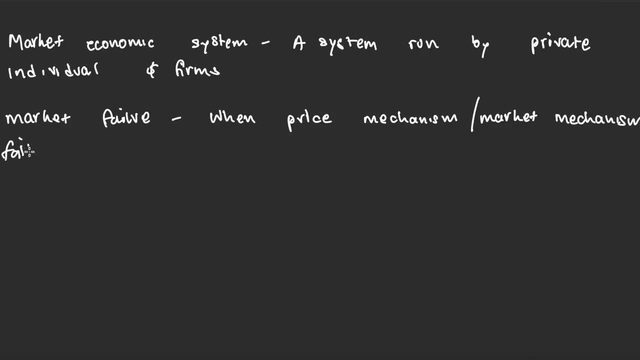 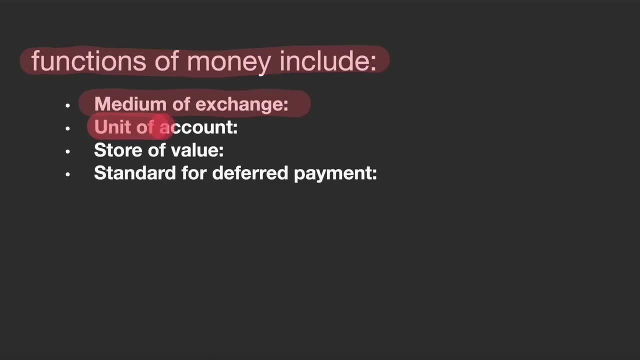 Market failure is simply when the price mechanism or the market mechanism fails to allocate scarce resources. With the mixed economic systems, this is run by the government. Functions of money include: medium of exchange. unit of account, store of value. standard for deferred payment. Characteristics of: 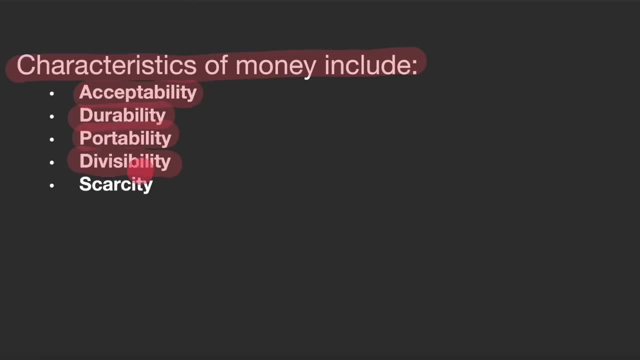 money include acceptability, durability, portability, divisibility and scarcity. We have two types of banks: commercial banks and central banks. We then have households and the inferences on households and borrowers With workers. factors which influence the choice of occupation are the level. 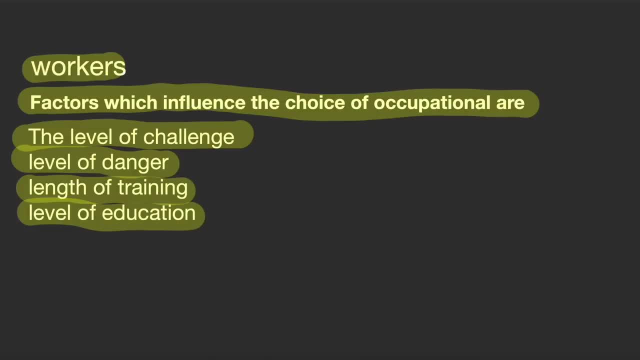 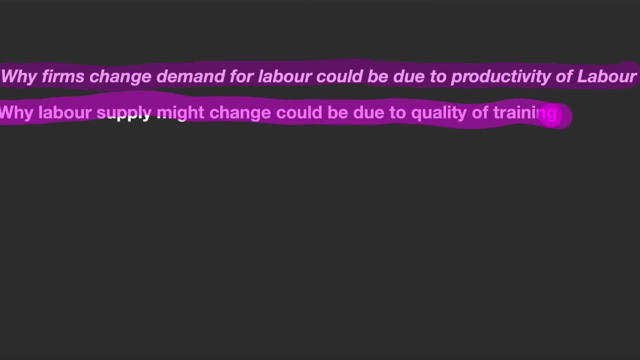 of challenge, level of danger, length of training and level of education. Why firms change demand for labour could be due to the productivity of labour, and why labour supply might change could be due to the quality of training. Factors that cause occupational wage differentials could be. 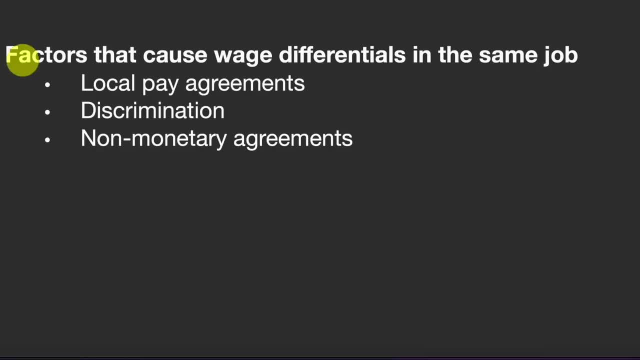 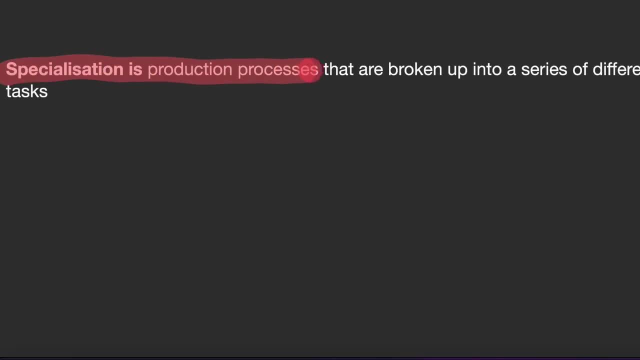 job satisfaction, fringe benefits, labour immobility. Factors that cause wage differentials in the same job could be local pay agreements, discrimination, non-monetary agreements. Specialization is production processes that are broken up into a series of different tasks. Trade unions are to protect the interest of its members concerning wages, benefits and 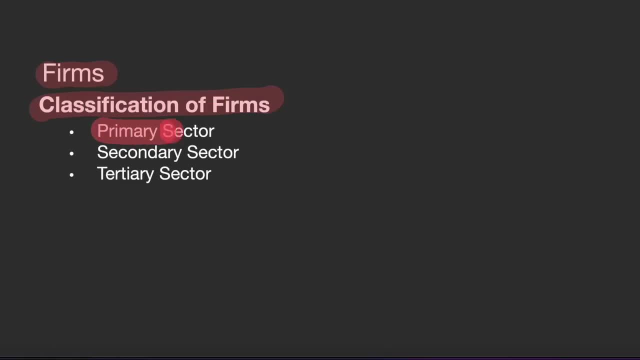 working conditions, Firms, Classifications of firms. we have private sector, secondary sector and tertiary sector. We then have the public sector and private sector, and the public sector is owned by the government and the private sector is run by individuals and owners. Merging is simply. 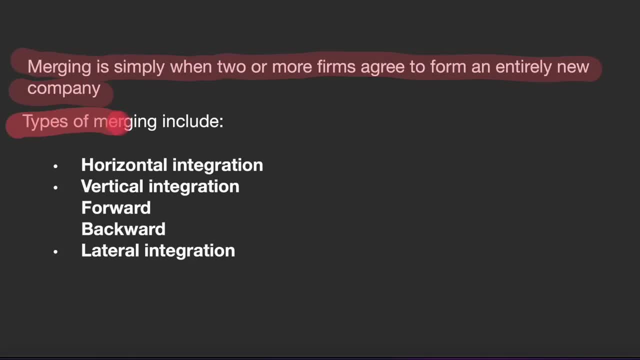 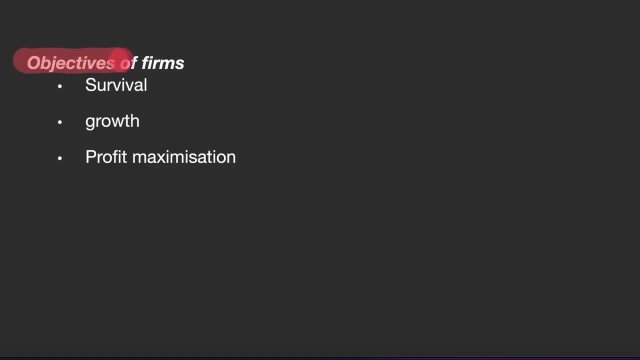 when two or more firms agree to form an entirely new company. The types of merging include horizontal integration, vertical integration, forward and backward and lateral integration. Objectives of firms are survival, growth, profit maximization and productivity. The market is a monopoly, and a monopoly is a company that dominates in the market. 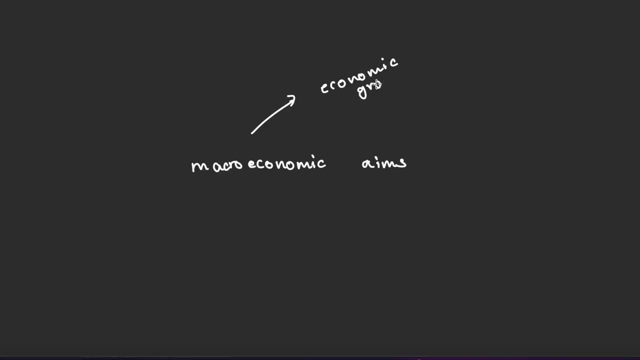 Let's start off with the macroeconomic aims of the government, which are: economic growth, low unemployment, low inflation and stable prices, balance of payment stability and redistribution of income. We then have three types of policies that the government uses to boost the economy, which are: 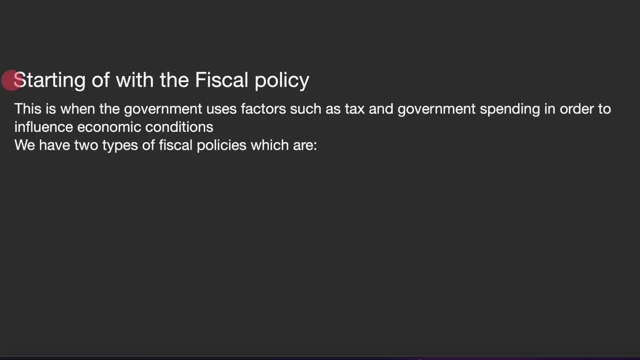 physical policy, monetary policy and supply side policy. Starting off with physical policy, this is when the government uses factors such as tax and government spending in order to influence the economic conditions. We have two types of physical policies which are: expansionary: physical policy which reduces inflation and economic growth. We have two types of physical policies which are: 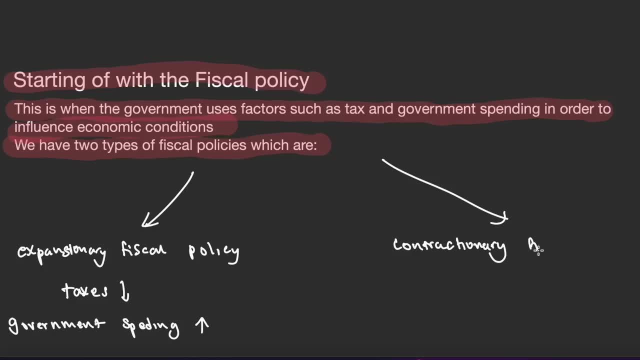 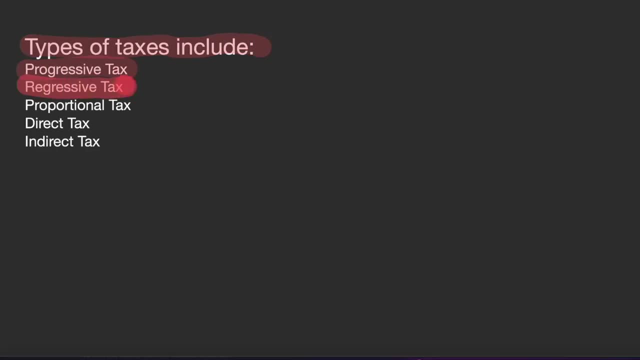 contractionary physical policy, which reduces the taxes and increases the government spending. We then have the contractionary physical policy, which increases taxes and reduces government spendings. The types of taxes include progressive tax, regressive tax, proportional tax, direct tax and indirect tax. Monetary policy: it is the use of interest rates to control the money supply and 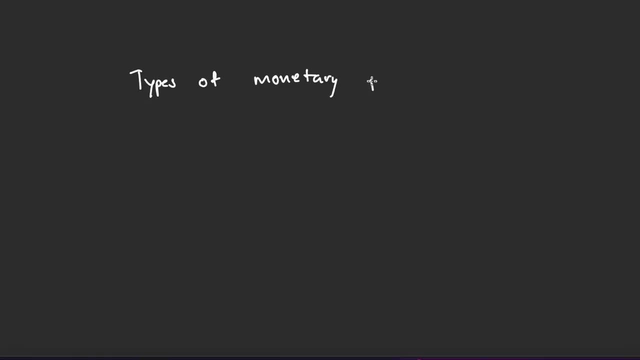 exchange rate to influence aggregate demand. We have two types of monetary policies, which are contractionary monetary policy, which is used to reduce price inflation by increasing the interest rates, and we have expansionary monetary policy, which is used during a recession and to increase employment by cutting interest rates. We then have supply side policies. 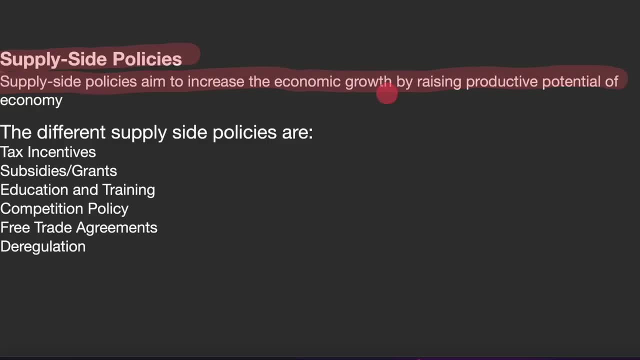 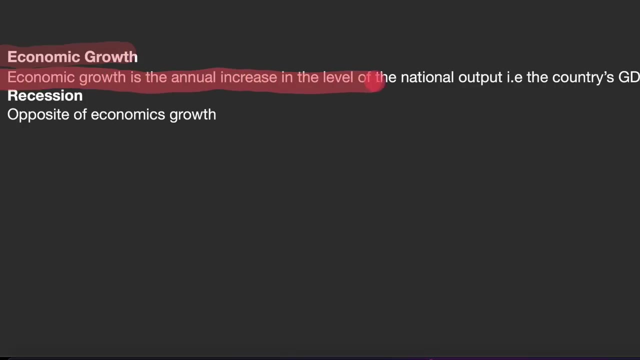 Supply side policies aim to increase the economic growth by raising productive potential of the economy. The different types of supply side policies are tax incentives, subsidies and grants, education and training, competition policy, free trade agreements and deregulation. Economic growth is the annual increase in the level of national output. 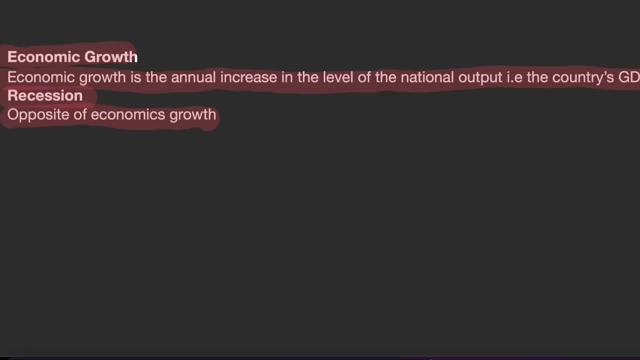 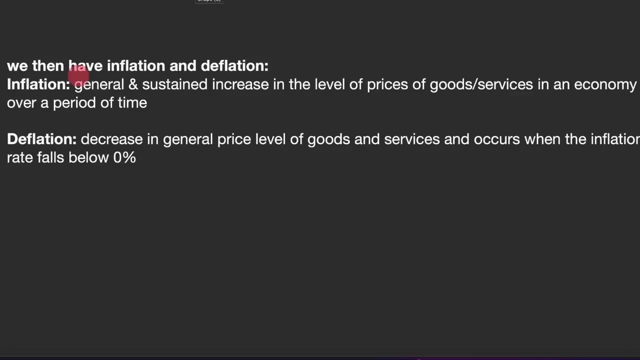 that is the country's GDP, and recession is the opposite of economic growth, of employment, include cyclic unemployment, structural unemployment, frictional unemployment and seasonal unemployment. We then have inflation and deflation. Inflation is the general and sustained increase in the level of prices of goods and services in an economy over a period of time. 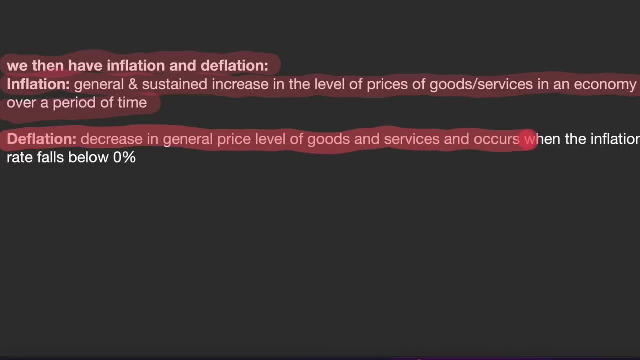 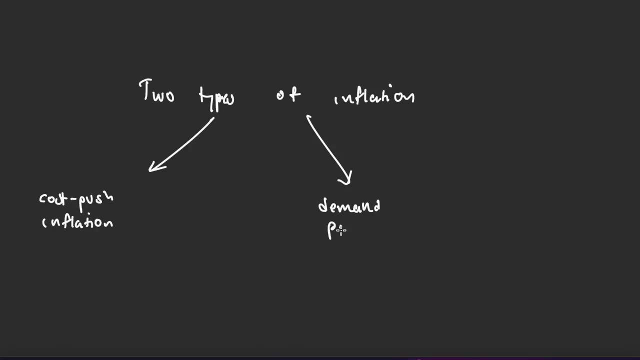 while deflation is the decrease in the general price of levels of goods and services and occurs when the inflation rate falls below 0%. We have two types of inflations: cost push inflation and demand pull inflation. Now, moving on to economic developments, We have living standards, poverty. 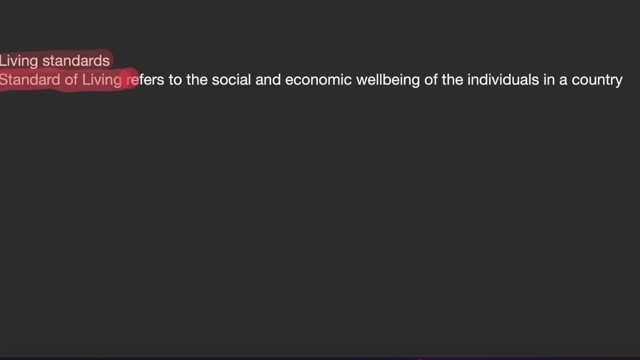 and population Living standards. Standards of living refers to the social and economic well-being of an individual in a country. GDP is the main measure of total value of all goods and services produced in a given period of time. With poverty, we have two types of poverty. 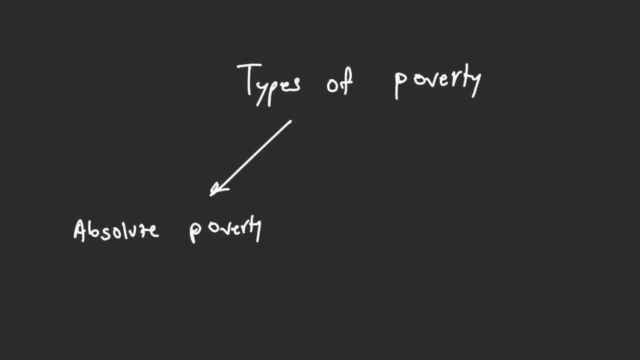 Absolute poverty, which are the number of people living below a certain income threshold or number of households that are unable to afford the basic goods and services. We then have the relative poverty, which are measures extend to which a household's financial resources fall below an 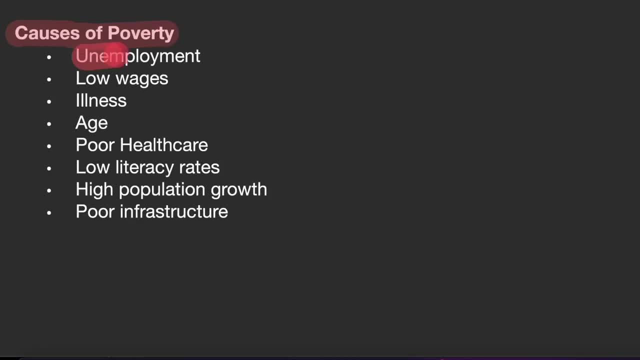 average income Level. The causes of poverty are unemployment, low wages, illness, age, poor health care, low literacy rates, high population growth and poor infrastructure. With population factors that affect population growth are birth rate, death rate, immigration and emigration. 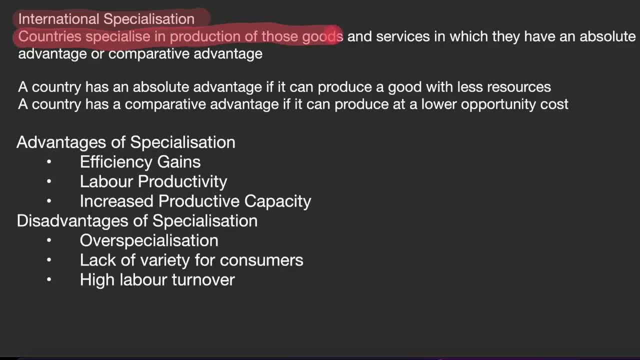 International specialization. Countries specialize in production of those goods and services in which they have an absolute advantage or comparative advantage. A country has an absolute advantage if it can produce a good with less resources. A country has a comparative advantage if it can produce a good with less resources. A country has an absolute advantage if it can. 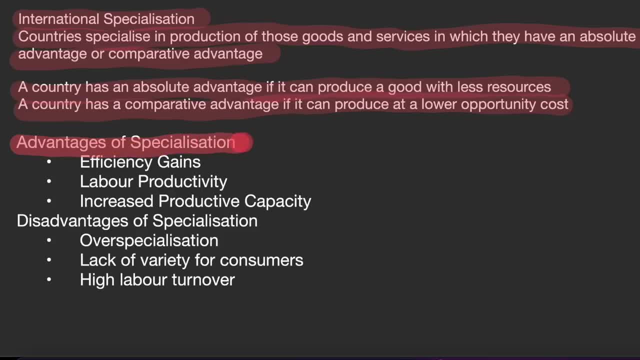 produce a good with less resources. A country has an absolute advantage if it can produce at a lower opportunity cost. Advantages of specialization are efficiency gains, labor productivity, increased productive capacity, And disadvantages of specialization are overspecialization, lack of variety of consumers, high labor turnover. Globalization, the process by which 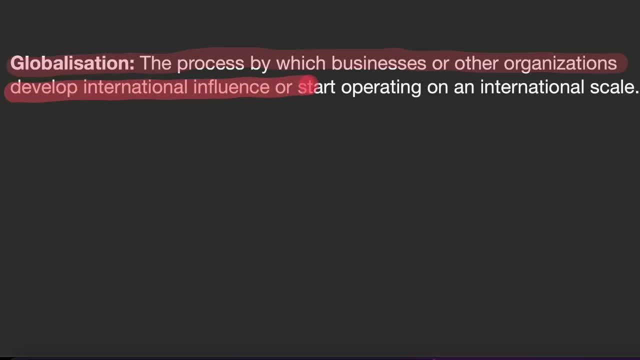 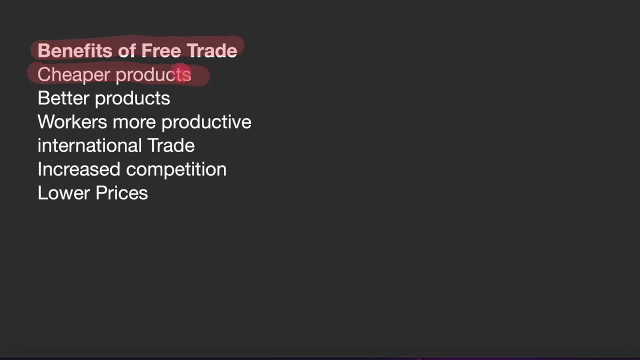 business or other organizations develop international influence or start operating at international scale. Multinationals operate in more than one country. The benefits of free trades are cheaper products, better products, workers, more productive international trade, increased competition and lower prices. With trade protection, we have tariffs.